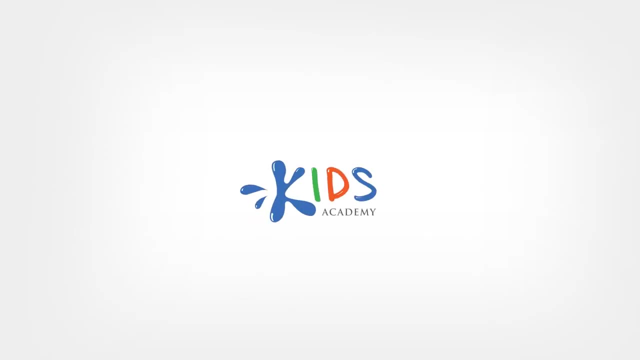 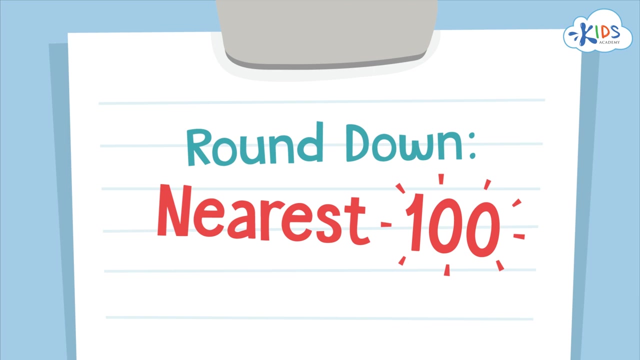 When we want to round a number to the nearest hundred, you have to look at the tens place to help you to decide to round up or down. I like to underline the place I'm rounding to the hundreds place and draw an arrow to the place that will tell me whether to round up or down the tens place, You always look one place to the right of the place you want to round to. So in this case we're rounding to the nearest hundred, so we'll have to look at the place to the right of the hundreds, which is the tens. The same rule applies when: 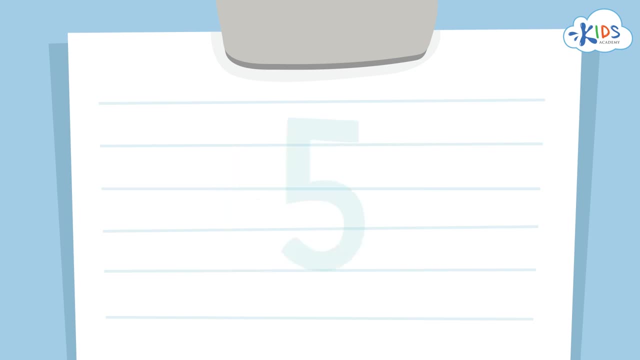 rounding to the hundreds place, as it does for rounding to the tens place. Five is the key number. If it's five or higher, you round up, but if it's four or lower you have to round down. You round the number in the hundreds place. 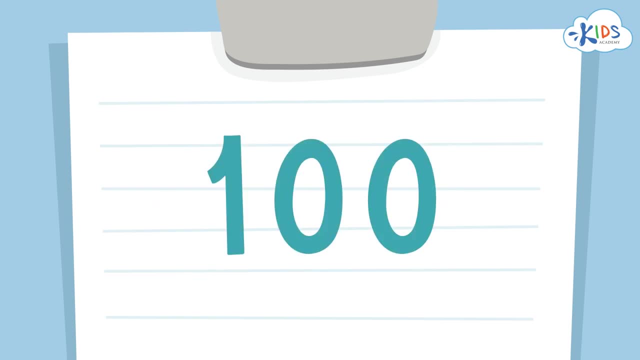 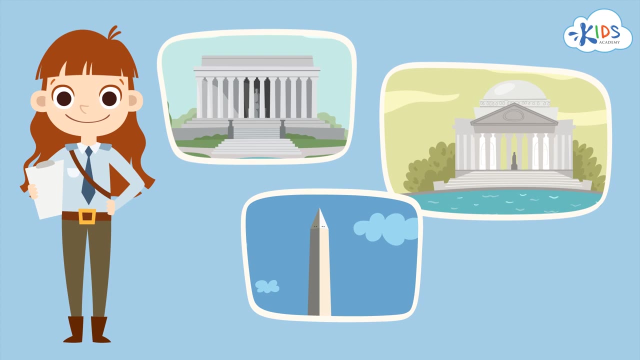 and make the numbers in the ones and the tens places zeros. Let's take a look at a real life situation that requires rounding and see how our rounding to the nearest hundred skills can come in handy. This park ranger wants to record how many people visited these landmarks by rounding up to the nearest hundred. Let's help her. 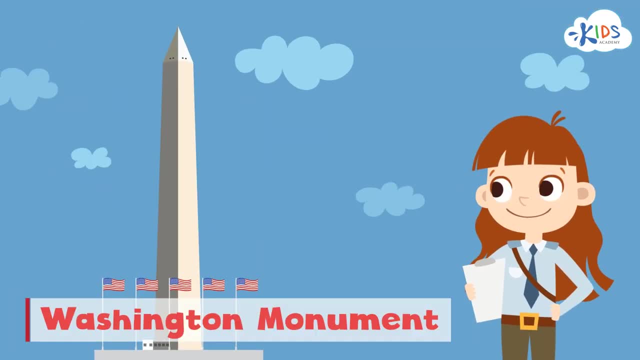 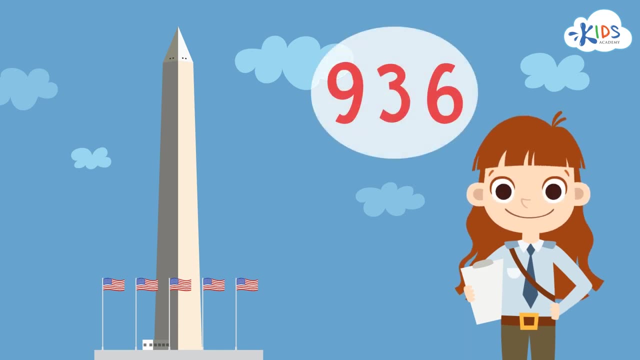 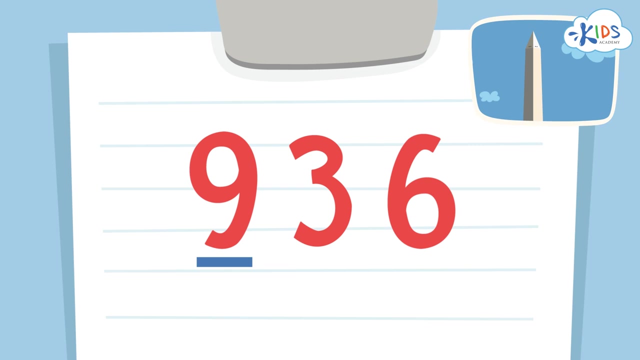 by rounding. First, we'll check out the Washington Monument, one of my favorite landmarks. According to the Washington Monument, 936 people have visited the Washington Monument. Now let's round this number to the nearest hundred. We'll use the strategy of underlining the. 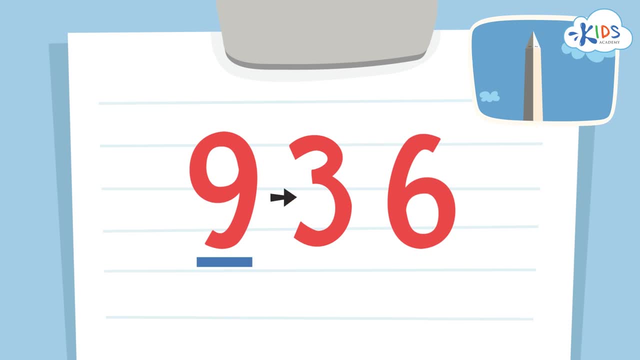 hundreds place and drawing an arrow to the tens place. so we know what numbers we have to look at. I see a three in the tens place. I know if it's four or lower we have to round down. The nine in the hundreds place is underlined. so we have to round down the 936 to 900.. I'm 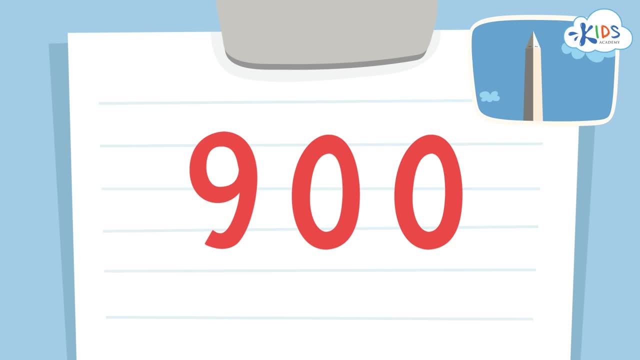 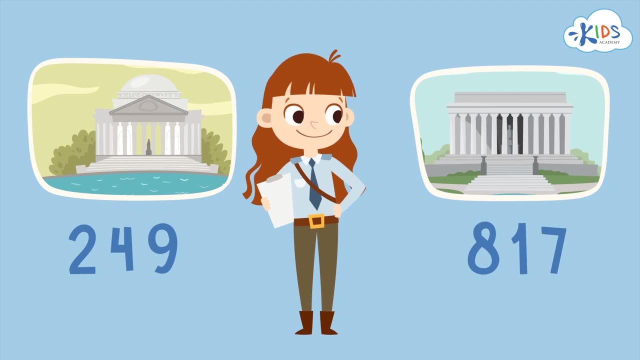 going to do that. When rounding to the hundreds place, the numbers in the tens and ones places become zeros. I'll leave you with a challenge. I want you to help the ranger round the next two landmarks' visitors to the nearest hundred. I'll give you some time to think, but if you 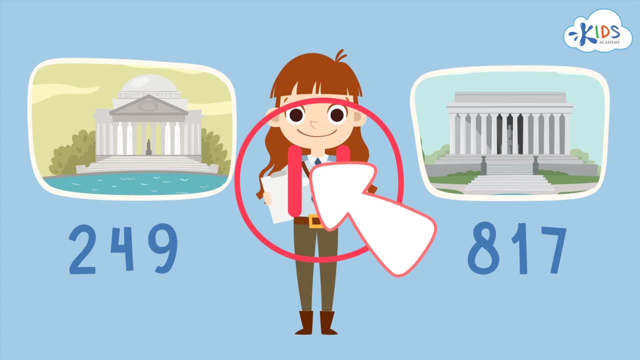 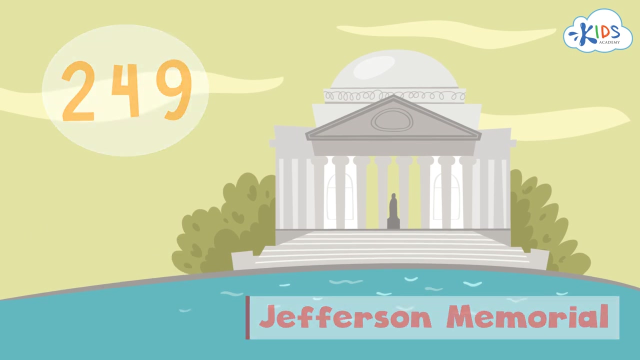 need some more time. you can pause the video and answer when you're ready. Okay, here's the answer. The Jefferson Memorial saw 249 visitors, so we're going to round 249 to the nearest hundred place. We'll use the strategy of underlining the hundreds place. 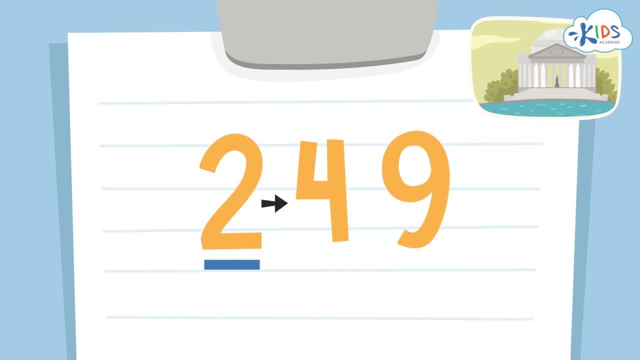 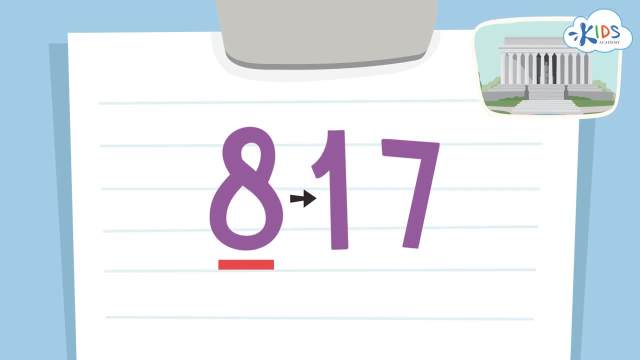 arrow to the tens place so we know what numbers we have to look at. I see a 1 in the tens place. I know if it's 4 or lower. we have to round down. The 8 in the hundreds place is underlined. so we have to round down from 817 to 800.. Remember. 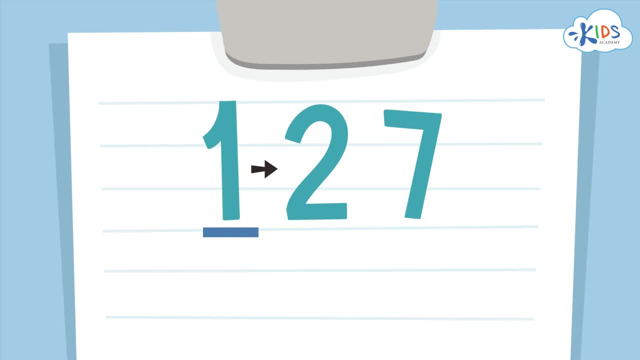 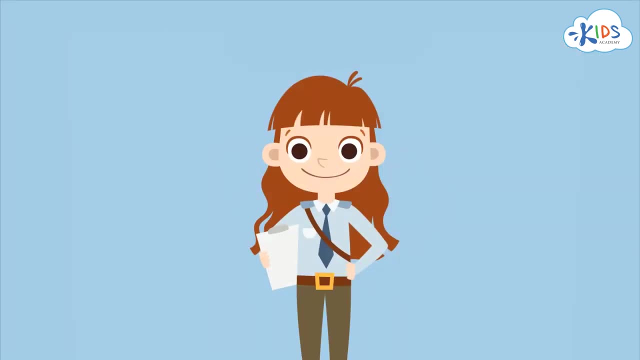 to look at the place of the right of the place that you want to round to and round down if you see a 4 or lower. Thanks for watching, boys and girls. We'll see you next time.